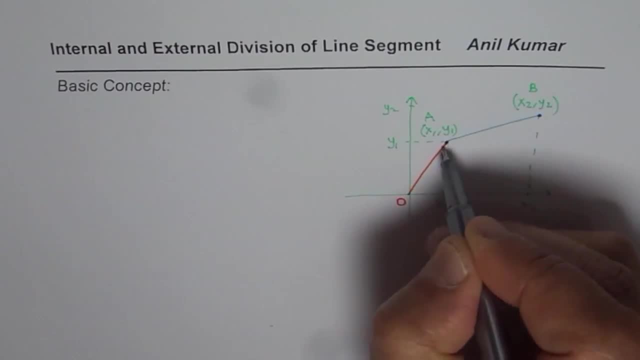 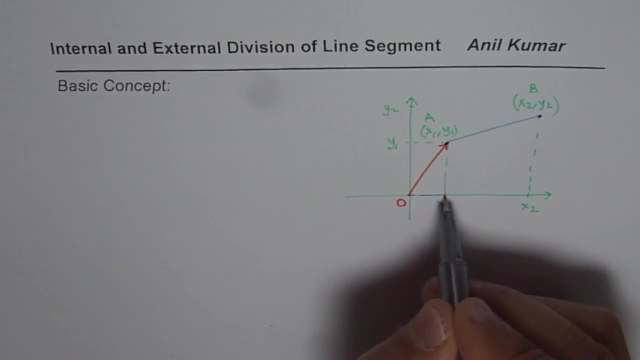 an O and from origin. If you want to go to point A, you move X units, X1 units along the horizontal axis and Y1 units along the Y axis to reach there. Similarly, if you have to go to point B, you have to go X2 units along the horizontal and Y2 units along the vertical line. 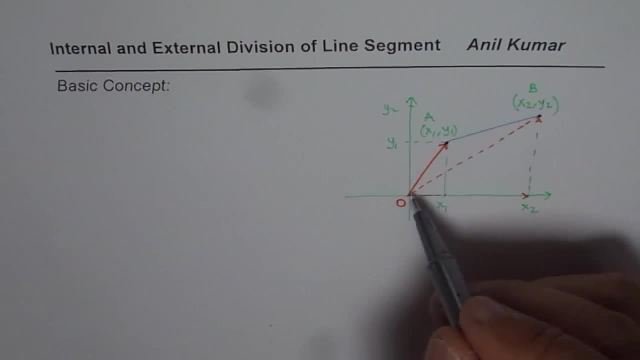 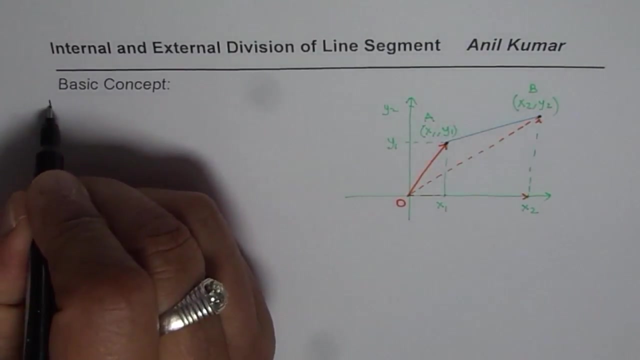 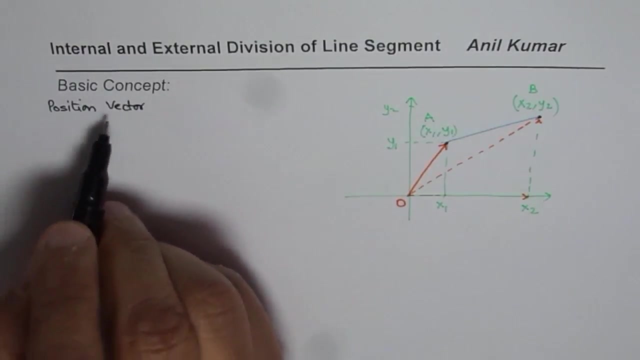 So then you reach point B. So sometimes we also refer these points as OA. So OA is position vector right, or we could say just position coordinates for the time being right. So if I use the word position right, so if I say position vector, some of you who are not doing vectors- you can say position coordinates right. 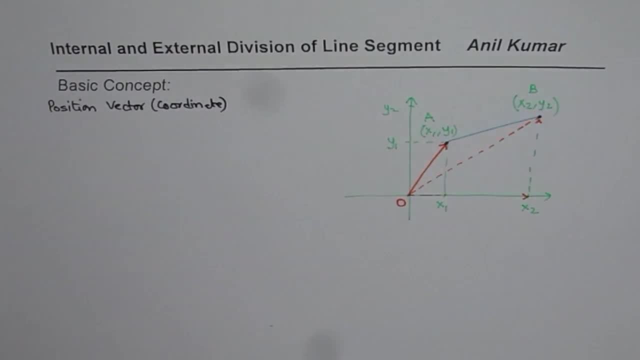 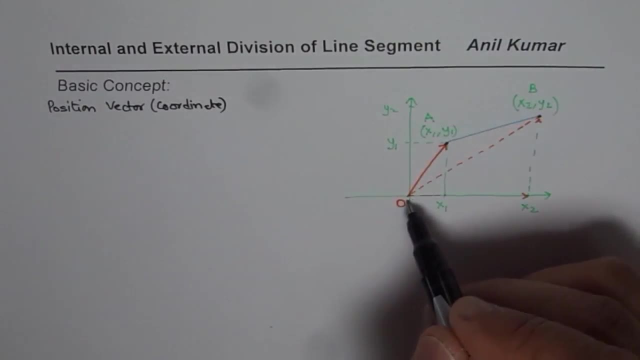 So that is what I am trying to say, right? So I am saying that OA is the coordinate point x1 by 1, right and OB is the position of B In our coordinate plane. right, OB just gives the coordinate points of B with reference to this coordinate plane, where origin is at 0, correct? 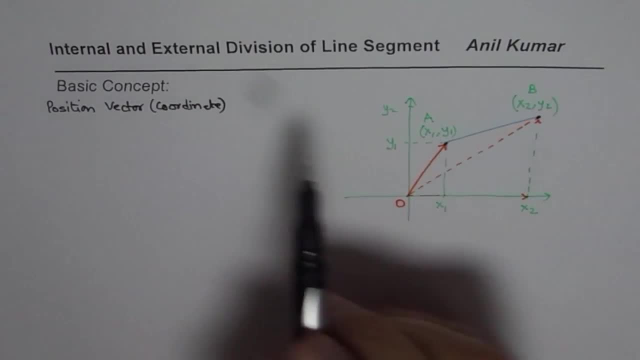 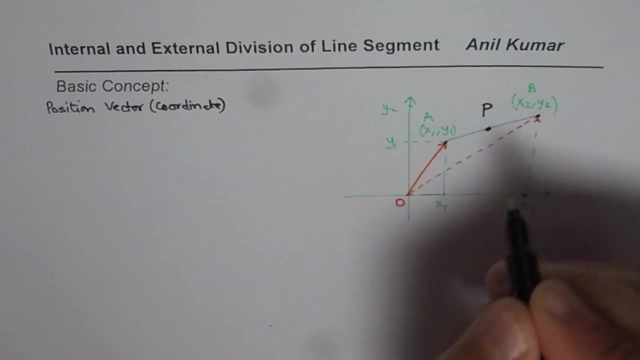 So that is what we are trying to say. Now let us talk about division of this line. We could have a point here. Let me call this point as P. Now this point could divide AB in some ratio, right? So let us say, this small portion which divides between A and B is small a and the one between P and B is B, right? 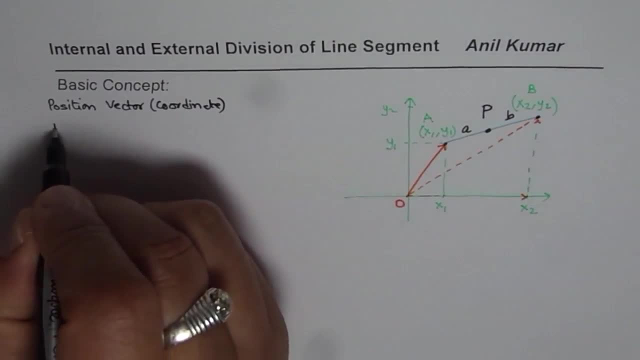 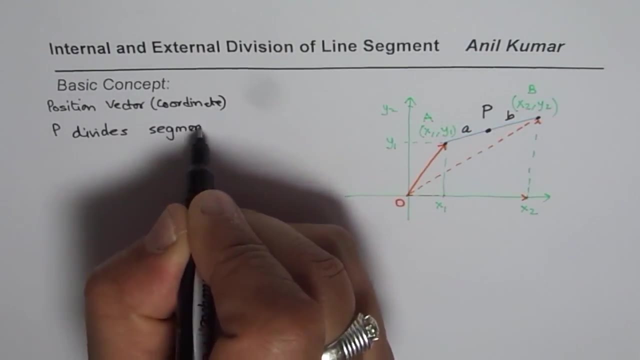 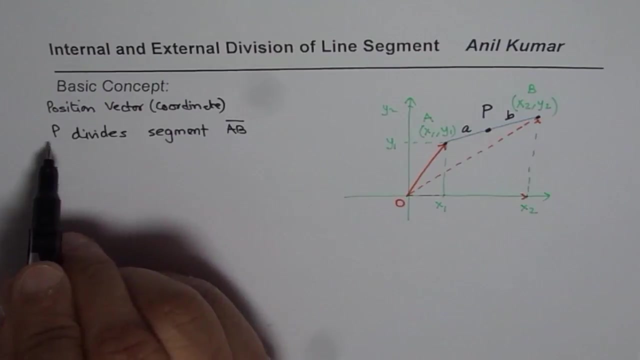 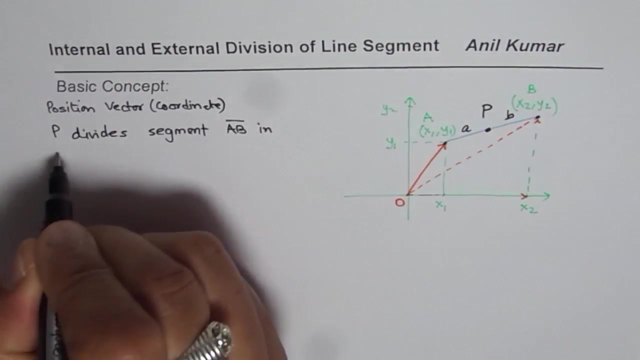 So in that case what we say is: P divides segment AB. Sometimes we may write a line over it saying segment AB. So we say P divides the segment AB in the ratio of A is to B, in ratio of A is to B, right. 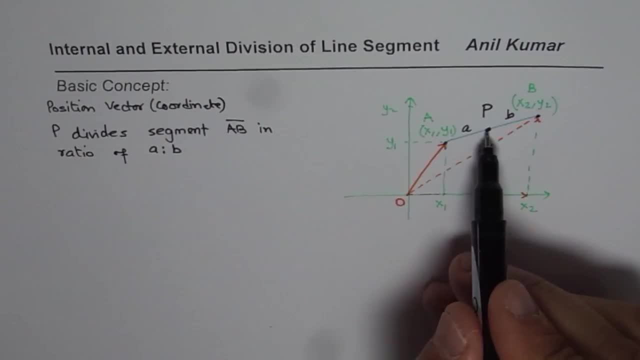 That is what we say. So here is a point: P which divides AB in the ratio of A is to B. Now, generally the questions are: what are the coordinate points, What are the coordinates of P right? So, given the values of A and B, how do we find P? 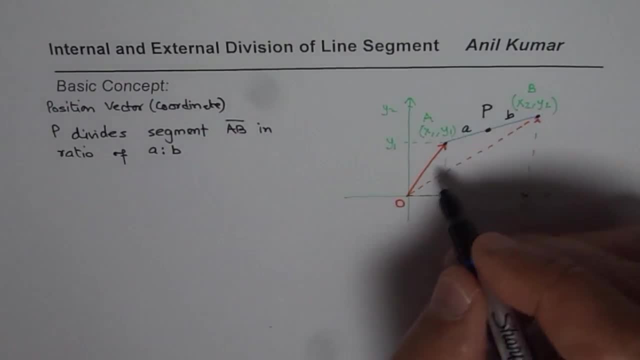 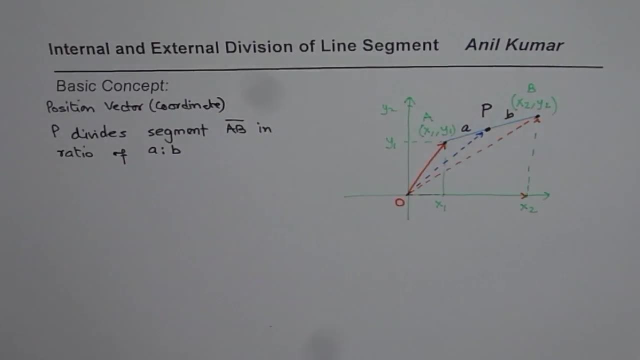 Or how do we find the position vector P right? So those who are doing vectors, they could treat this as position vector P. Now the formula for this is proof of this formula is given in another video, But here I will give you the formula so that those who are using coordinate geometry can also use the formula right. 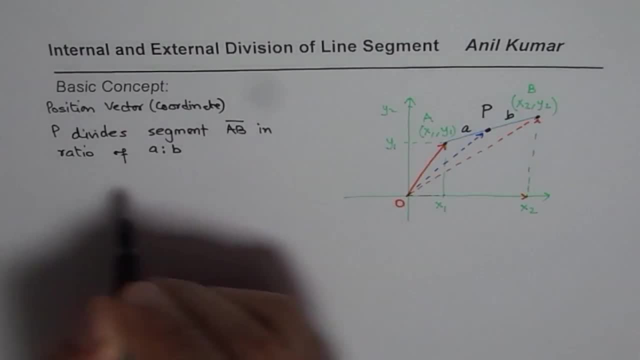 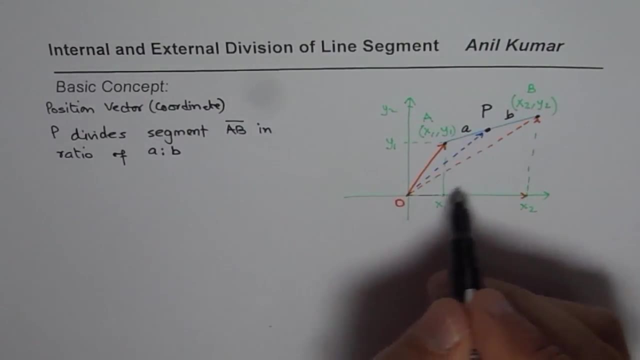 So we say the position vector of P. You could write O to P also. If I say O to P, that means I am going like O, this value X and Y. So that is how we get X and Y coordinates right. 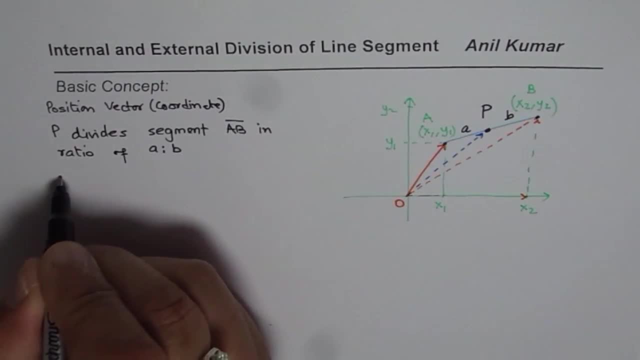 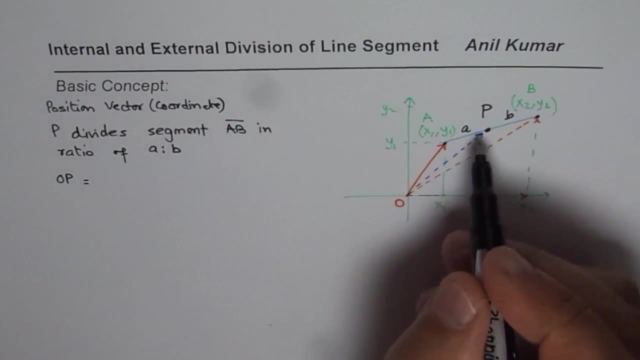 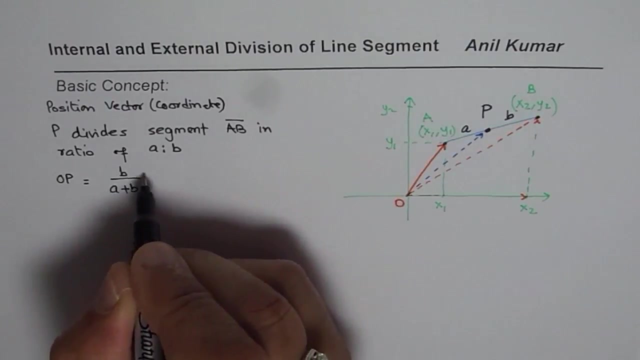 So let me write here as OP, okay. So the position vector P will be equals to the ratio in which it divides B over some of these two, B over some of A and B times the position vector of A Which I am saying OA right. 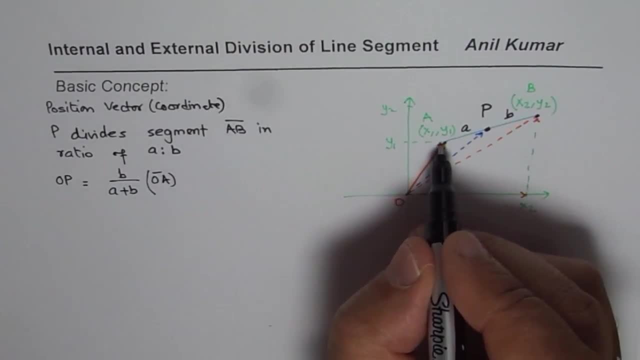 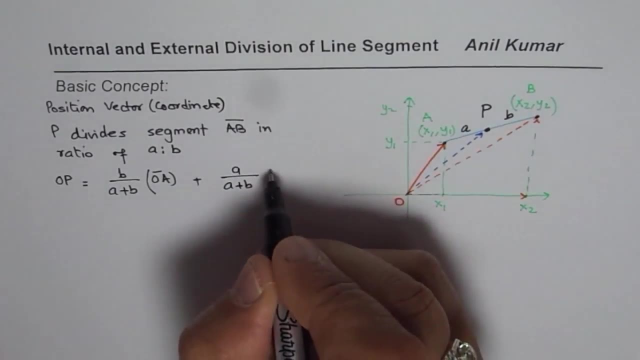 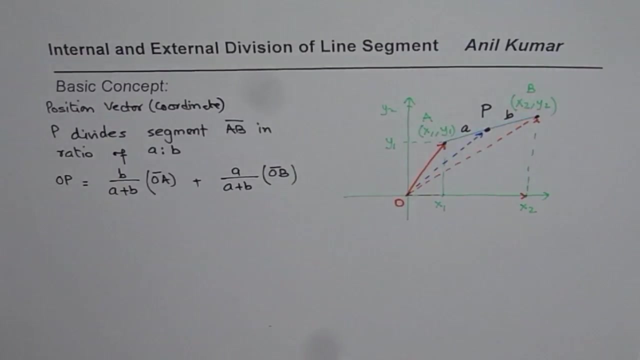 That is the one value. And then we add to this A of A plus P, the position vector of B. Let me write OP here, right, Okay, So that is how we get coordinate points of B, right? So what I am trying to say here is that if I could select- 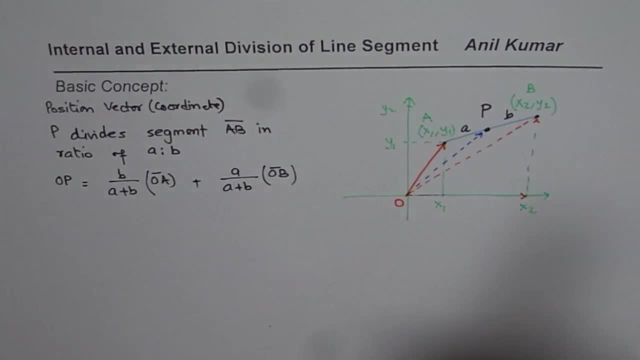 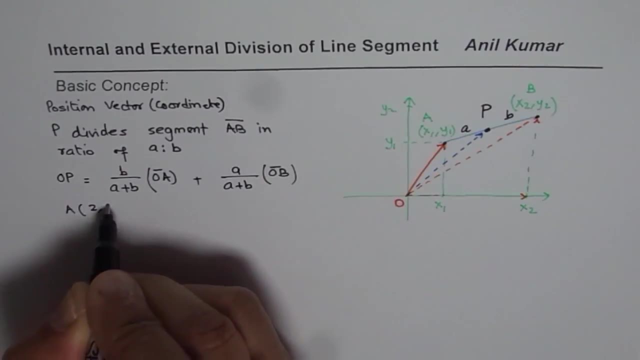 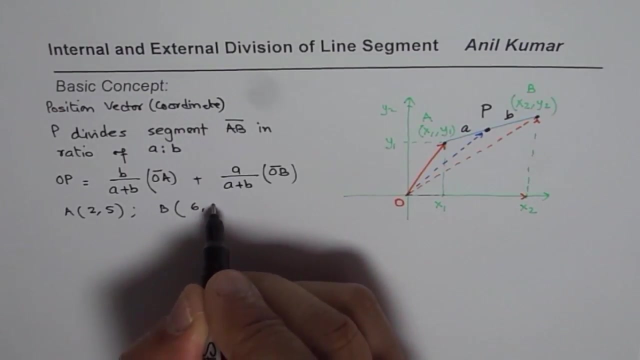 any point in general. for example, let us take point A, as let us say: point A is for us, 2,, 5, okay. And point B, as let us say 6,, 12, okay. So these are my two points. 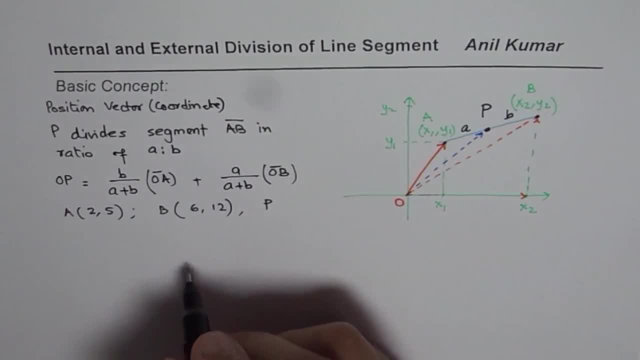 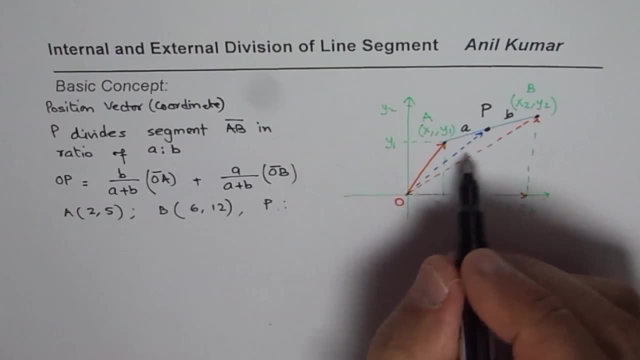 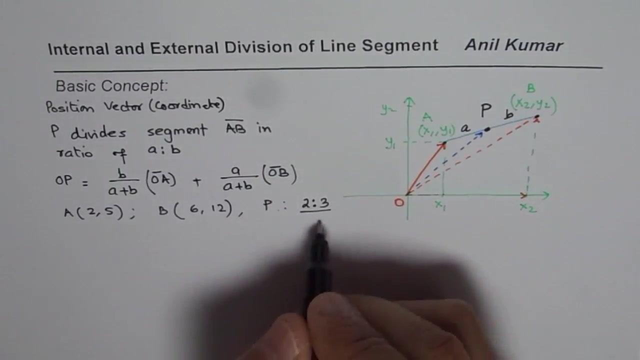 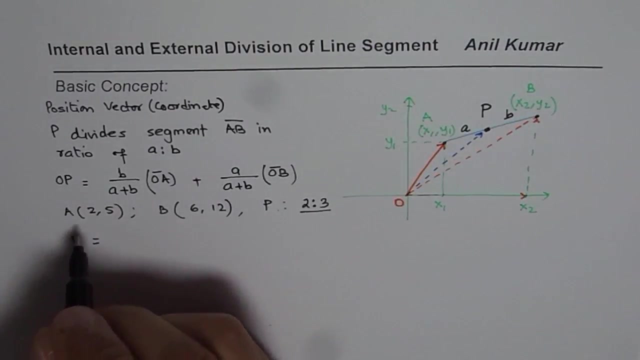 And we need to find point P which can divide AB in the ratio of, let us say, 2 is to 3.. So P divides in the ratio of 2 is to 3, okay, In that case coordinate points of P can be found as equal to. so I am not writing OP. 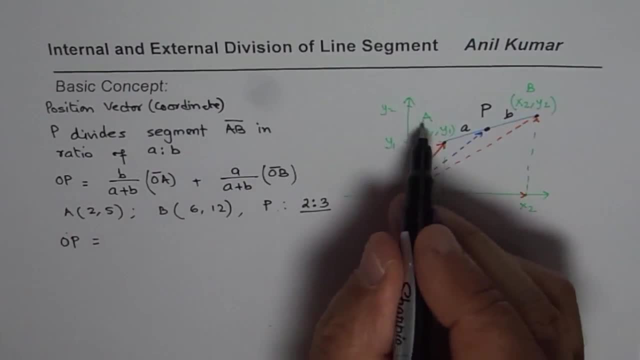 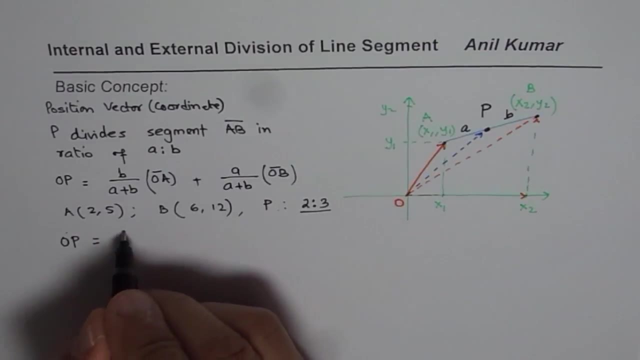 I could write OP also. OP gives position value which is in terms of X and Y, So B, B, is this value 3, right? So I write 3 over 2 plus 3.. Okay, Okay. 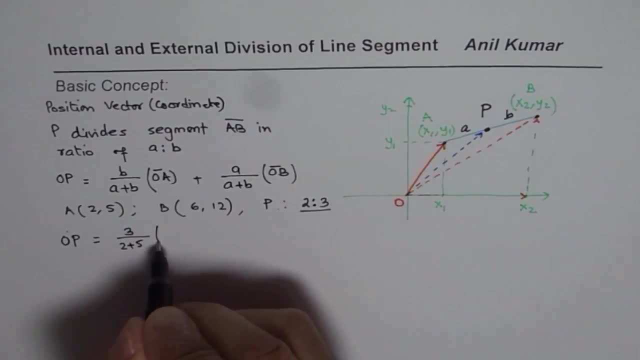 Okay, Okay, 2 plus 3, which is 5, times coordinate points of A, which is 2, 5.. So 2 is the X value, 5 is the Y value plus 2 over 2 plus 5, times coordinate points of. 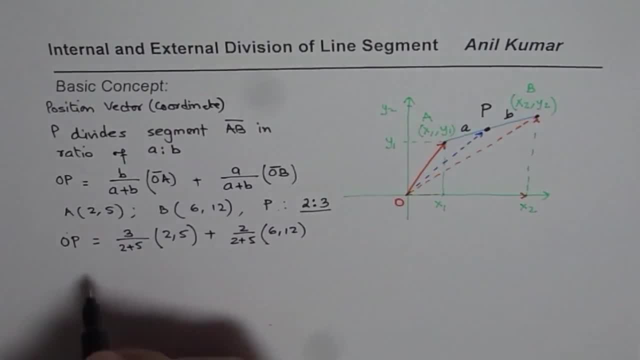 B, which is 6, 12, correct. So then what you can do is you can do 3 over 7, times 2, 5, plus 2 over 7.. So you can do 3 over 7, times 2 over 7, times 2 over 7, right. 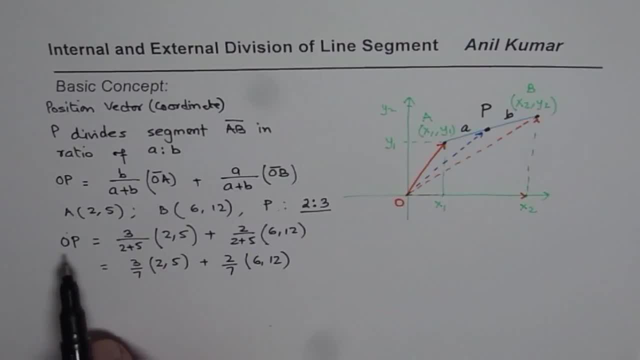 So you can do 3 over 7, times 2 over 7, times 2 over 7,. right Now to get the coordinates of P. these are the X values and those are the Y values. So you add the X values and the Y values, correct. 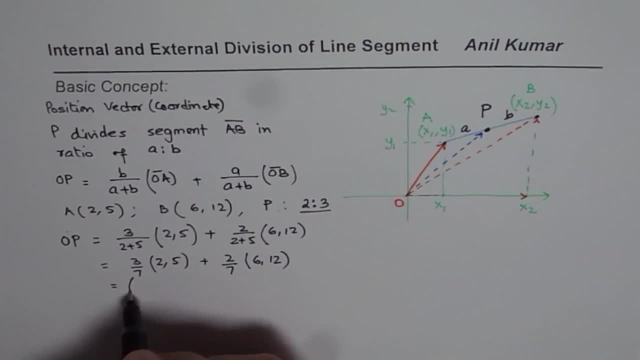 So you could write this as big brackets: So 3 times 2 is 6,, right, 6 over 7, and here we will add these X values. These are the X values, right? So I am adding these X values after multiplying by these numbers. 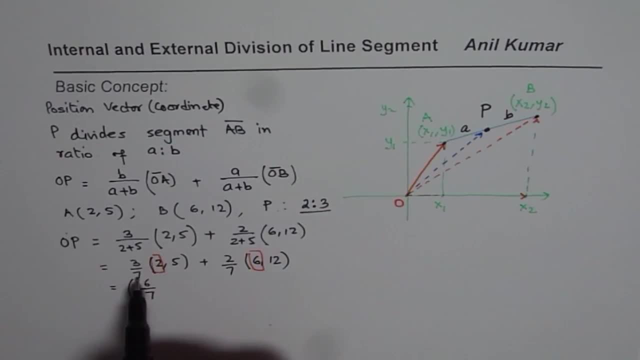 So it will be: 3 times 2 is 6, 6 over 7, and here 2 times 6 is 12,, so 12 over 7.. These are my x coordinate values, and the y coordinate values will be 3 times 5, 15 over 7, plus 2 times 12, 24 over 7.. 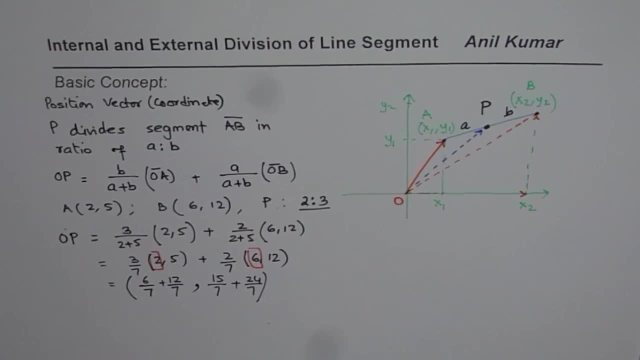 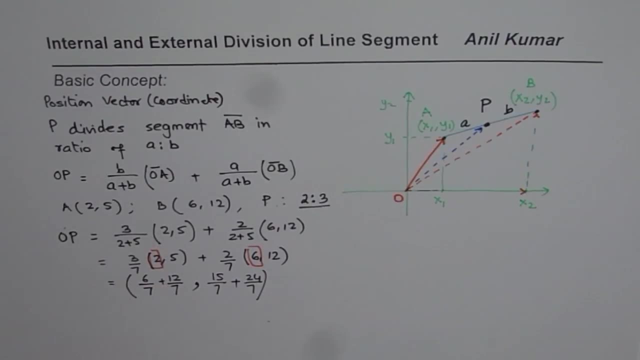 Do you see that? So that is how I could get my x and y coordinate points of P using this particular formula. You get the idea right. So of course, you could simplify this and say: 6 plus 12 is 18 over 7, and 15 plus 24 is 9 and 39 over 7, right. 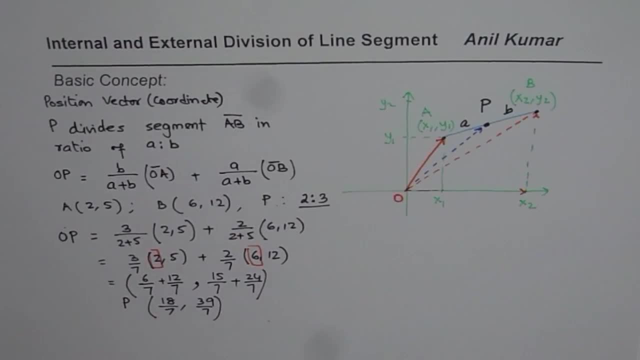 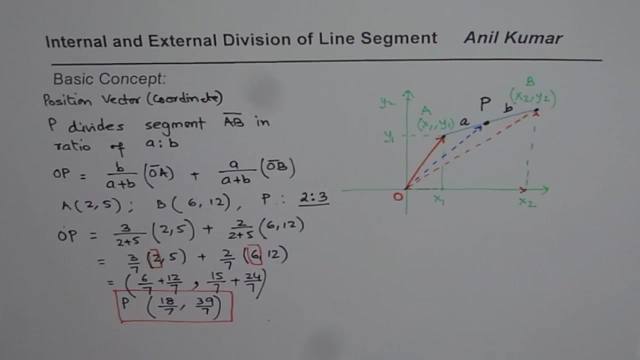 So those become coordinates of point P, right? So even if you write straight away just point P, it means coordinate points of P, right? So that is how we could actually calculate The coordinates of a point which divides. Now, whenever point P is within A and B, we say this is internal division. 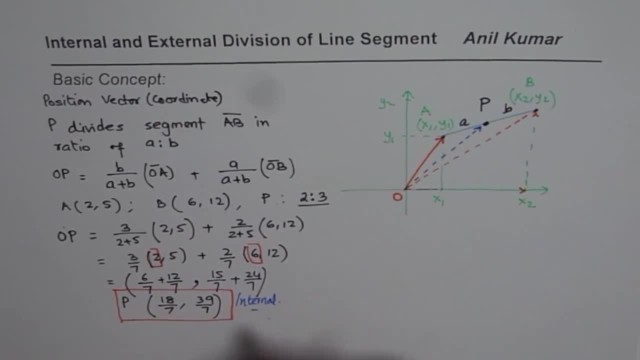 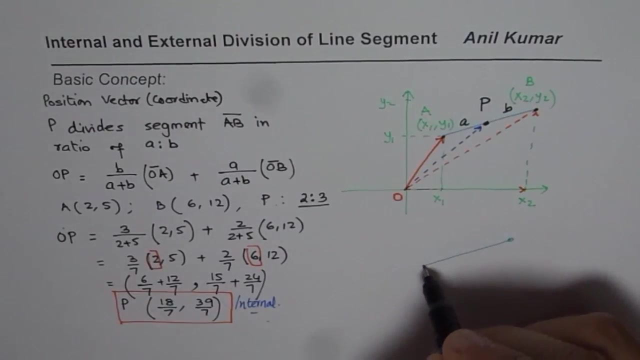 So it is internal, Since the point P is between these two points, correct? However, you could have external division of a line segment also. Now let us consider another line segment, right? So let us say these are my two points. I am not taking coordinates and I am not doing the calculation. 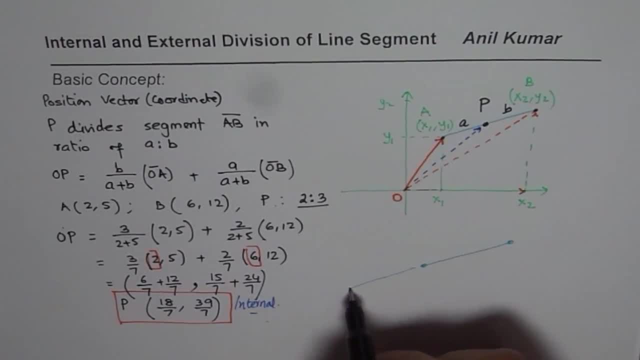 But I am trying to explain you the concept, So I will just extend this line a bit. You will understand why. So let us say these are my points A and B, And I have a point P, this time not in between them, But I think it is on the left side of A right. 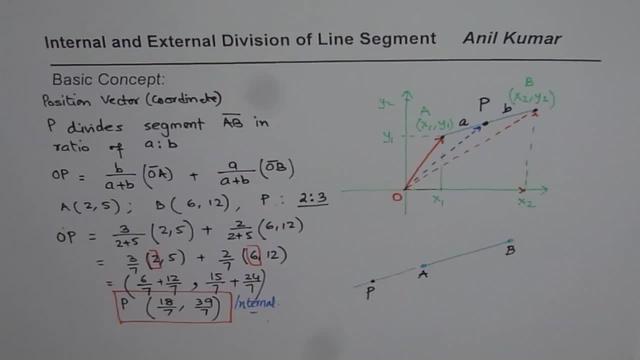 So let us say, this is my point P, which divides them into, let us say in the ratio of, let us say 1, 2.. Since I have moved from A 3 units left, I will call this as a ratio of: minus 3 is 2.. 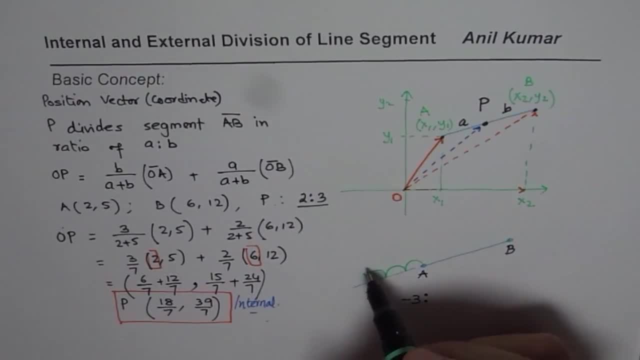 And see how many units I have to go from P to B. So it is like, let me use another ink. If I am going from P to B, then in this case it will be 1 unit, 2 unit, 3 unit, 4 unit, 5 unit, 6 unit, 7 unit. 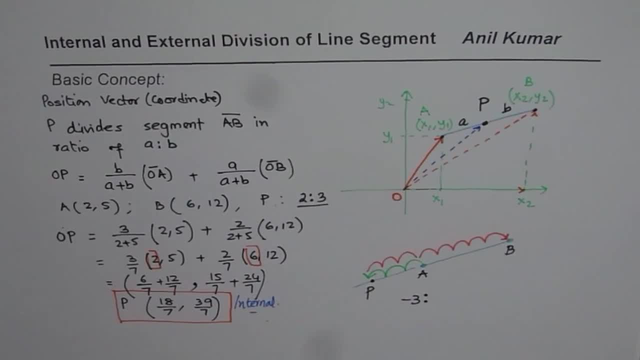 And let us say 8 units, right? So the ratio will be Minus 3 to 8.. So if the ratio which P divides A, B is minus 3 to 8, then it means it is external division, right. 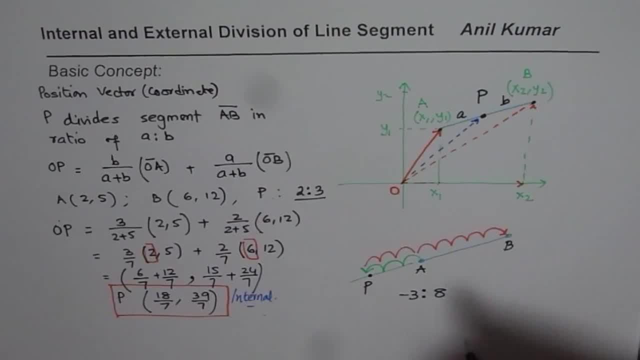 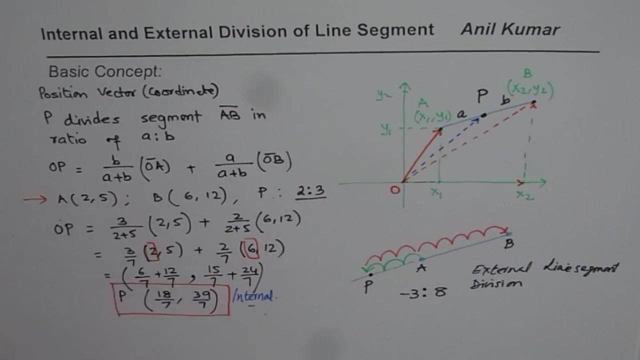 So this case, when P is not between A and B, we are talking about external line segment division. So in this case, point P divides A and B in the ratio of minus 3 is to 8.. Now, as an exercise, you can use this formula and find point P which will divide line segment given to us which we calculated earlier with, let us say, the line segment. is this one joining point A and B?